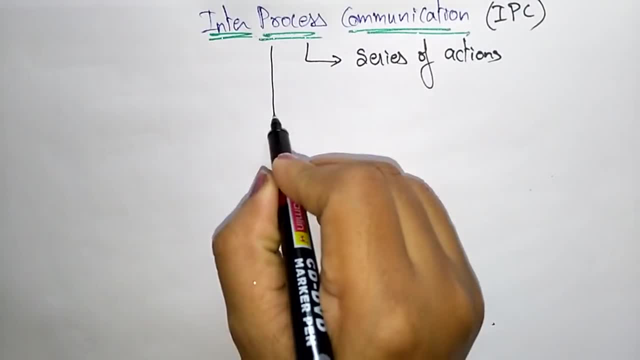 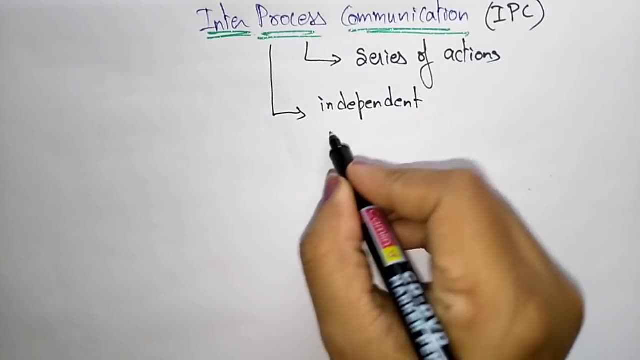 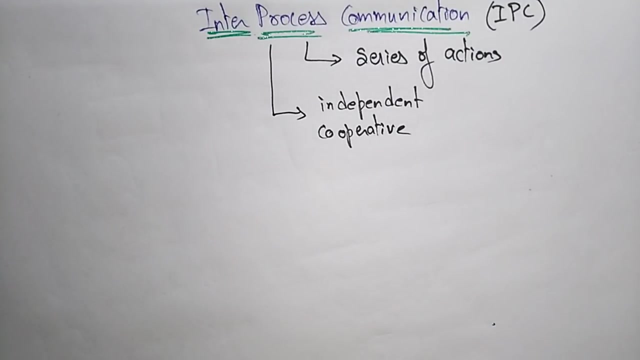 system may be a process within a system may be it is independent or cooperative. So a process may be independent or cooperative within a system. Suppose if it is an independent. suppose a process is an independent: it is not affected by execution of other process not affected. 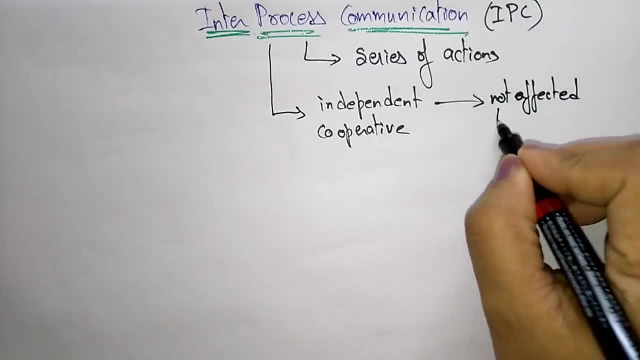 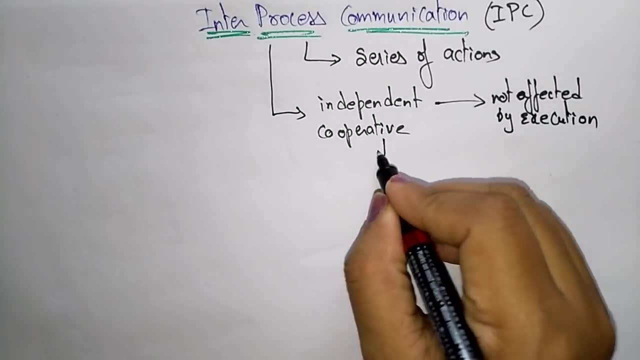 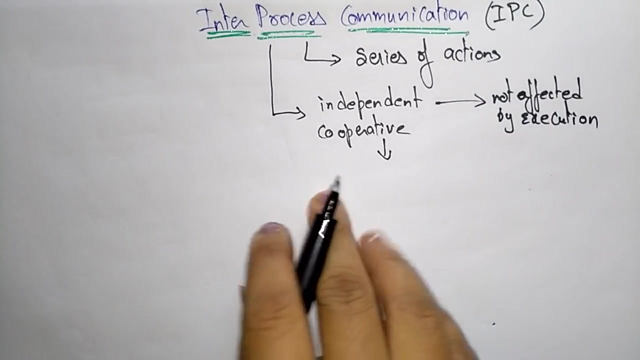 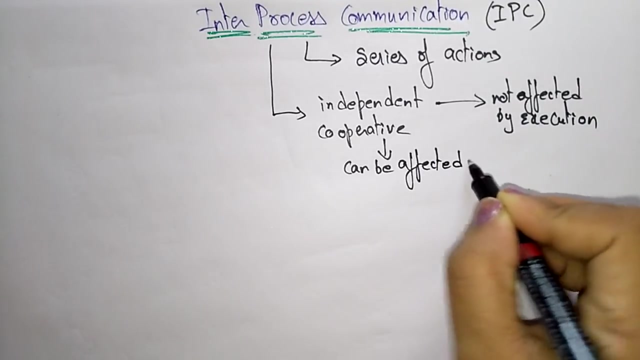 by execution of other process, By execution of other process. if it is a cooperative, so whatever the process that is taking place within the system. So if it is a cooperative, then compulsory, it is affected, it can be affected, It can be affected by other executing program. 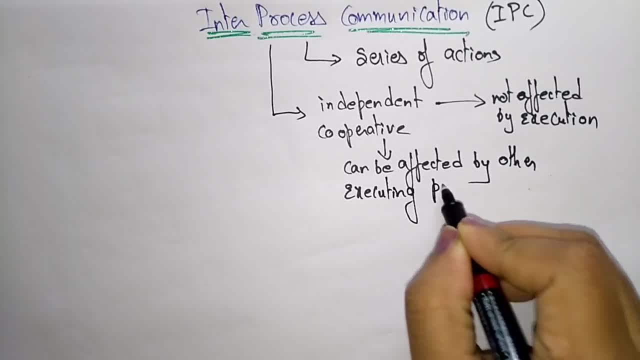 other executing program. Okay, so this process is nothing, but it is a series of actions that taking place while executing any program. A process can be independent or a cooperative. Suppose if the process within a system is an independent to each other, then it will not affect by execution of any process, because those all process will be independent to each other. 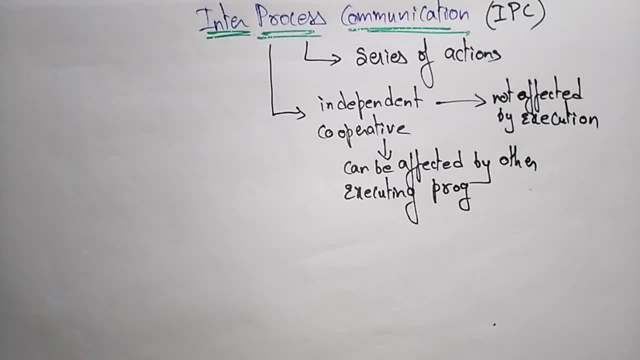 It is cooperative, So all the process will cooperate with each other. So all the process will cooperate with each other. So all the process will cooperate with each other. to each other, then compulsorily it will be affected by executing the other program, if one 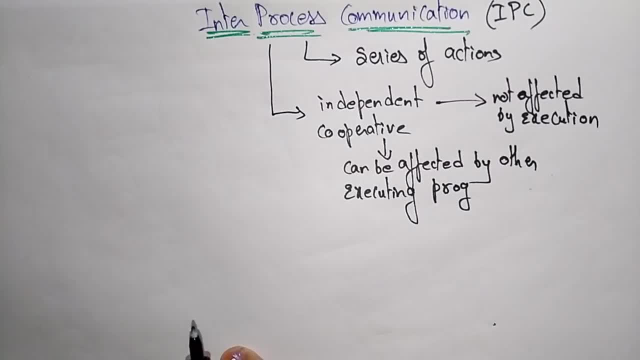 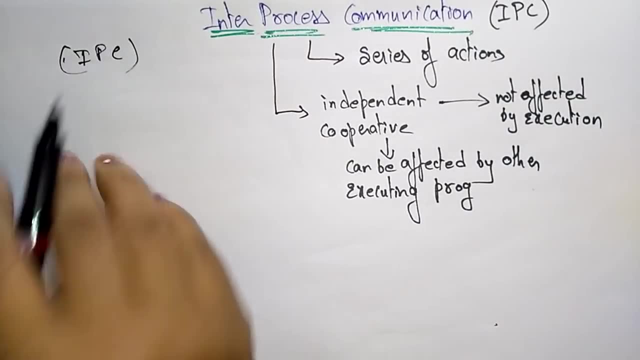 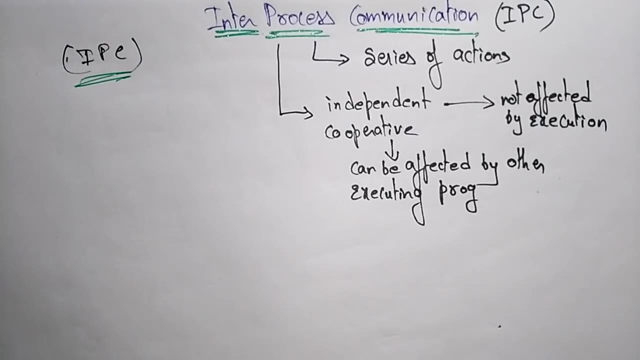 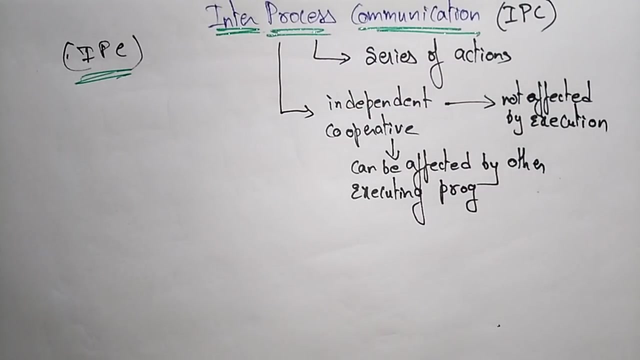 program is executing, it will be affected by other process. okay, so let us see this inter process communication. so what is this ipc, inter process communication? so actually, this inter process communication is a mechanism which allows processor to communicate with each other and to synchronize their action. so we call it is a mechanism. so it is a mechanism allows. 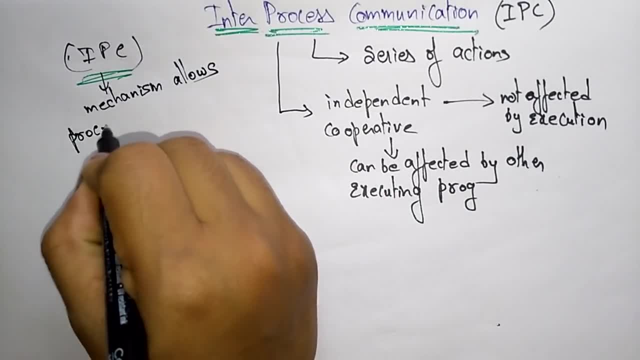 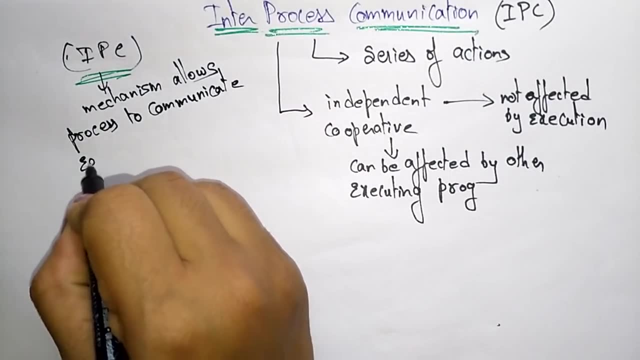 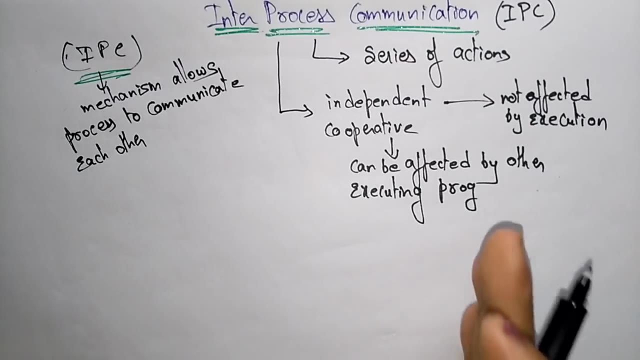 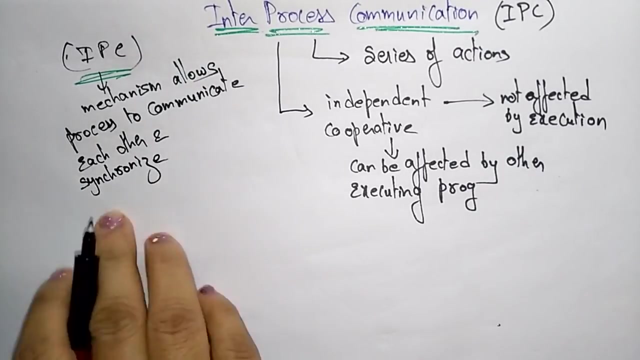 process to communicate, to communicate each other. so, whatever the process that are in the system, they can communicate with each other and they synchronize their actions. okay, synchronize their actions so that you call it as inter process communication. so this communication is nothing, but it is a method of it is in cooperation. so i already said that process. 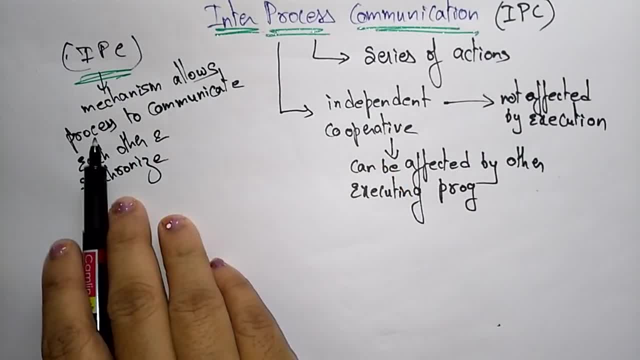 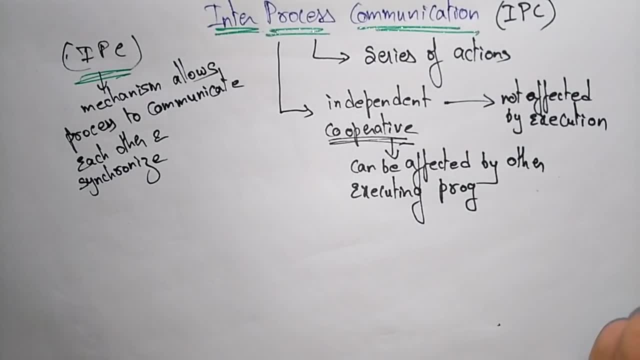 is a cooperative or independent. so if you take inter process communication, it should be compulsory. it is a cooperative, a cooperation with, between, uh is there between the processor. so inter process communication is a mechanism allows process to communicate and communicate each other and to synchronize their actions. okay, so let us see why we use ipc. so i said inter process communication. 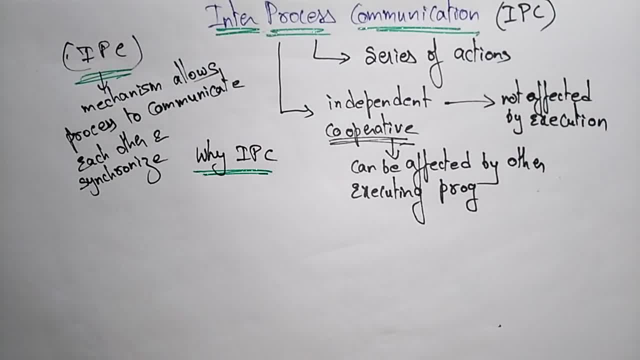 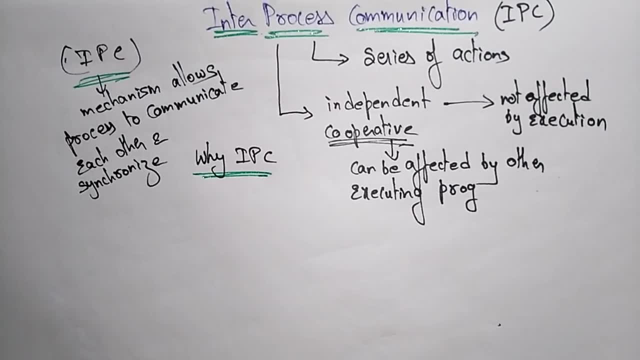 will be used to communicate all the process with each other and to synchronize their data. so why we are going for this ipc. is it required to use ipc within in the system? yes, so why we are using this inter process communication? so the first one is information sharing. is there? 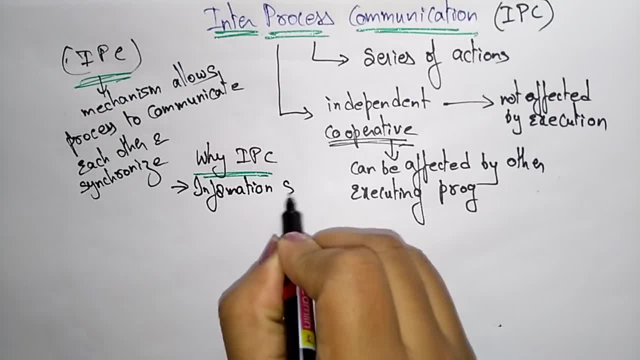 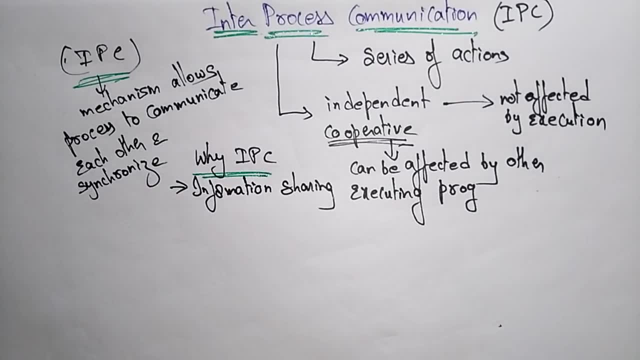 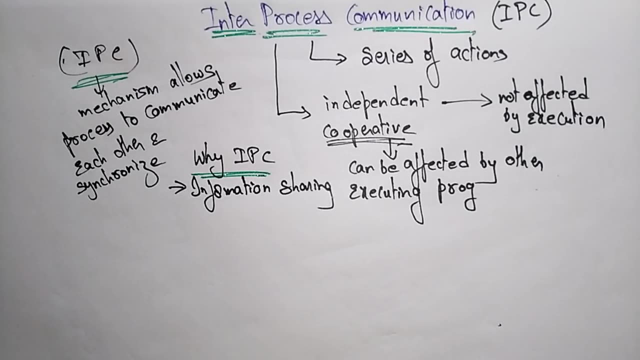 information sharing. so there is a information sharing will be there from one process to another process. suppose the process may be present within your system or within another system. with the help of networking they will be communicated. so if you use inter process communication, there is information sharing will be there and resource sharing. 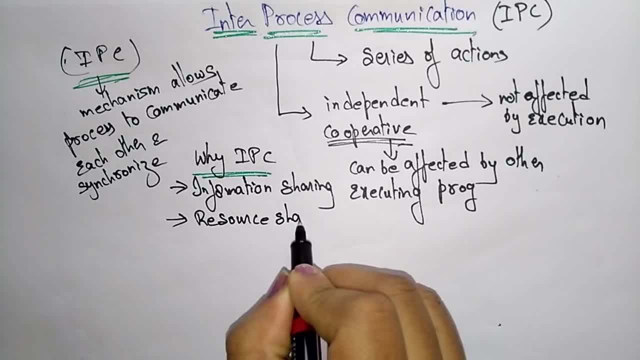 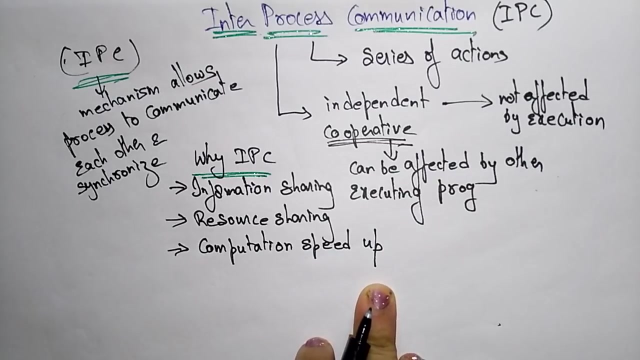 so, even though not only the information, you can share the resource also within the system or outside the system, if you use inter process communication, resource sharing. next, computational speed will be increasing, computation speed up. so computation speed up is also increase if you use limited resources, if those resources will be. 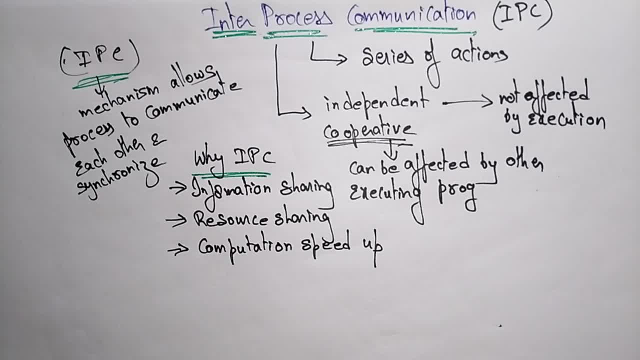 sharing by other process, also with the help of cooperation, then obviously the computation speed is also increase. synchronizing, synchronize, synchronization, so synchronization here itself with other process by means of same some of us, okay. so synchronization will help to communicate each process one by one, each other, sorry. so it synchronizes the data and it's having the modularity. 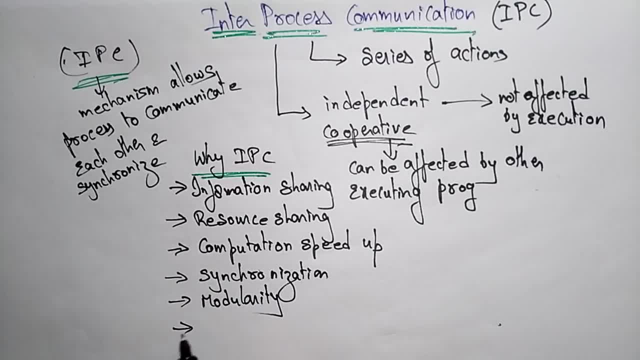 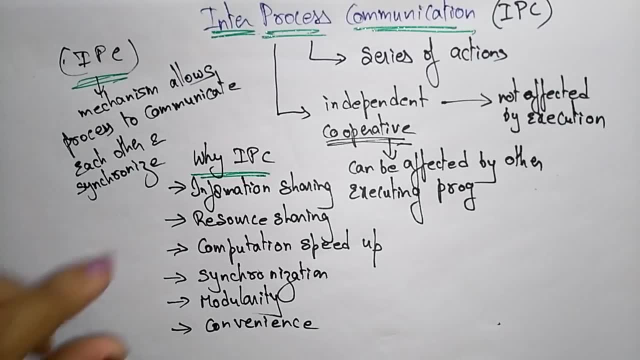 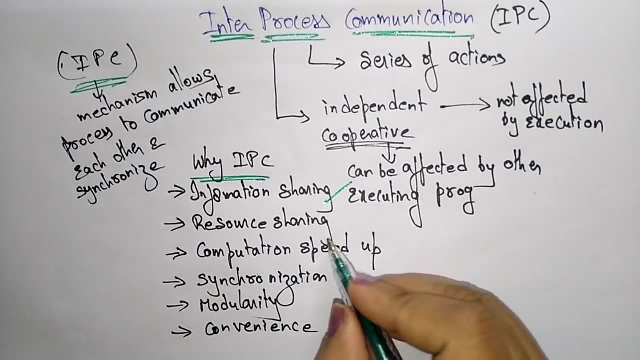 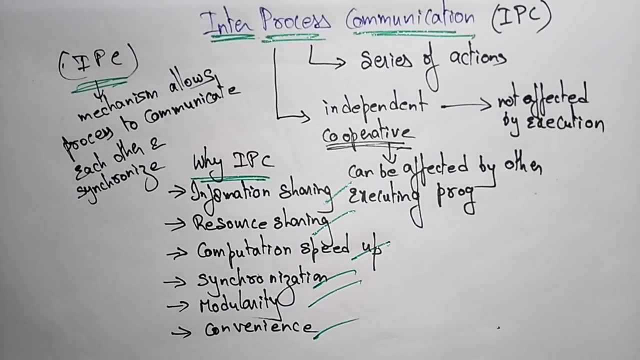 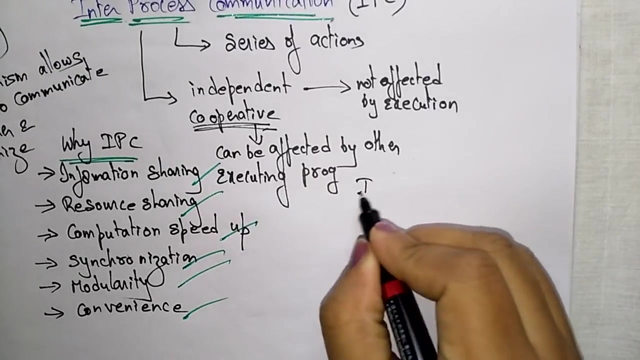 and it is convenience to use inter process communication. okay, so for these reasons, we are using this inter process communication: information sharing, information sharing, resource sharing, computational speed up, synchronization, modularity and convenience. okay, so next coming to the inter process communication mechanisms. so what are these IPC mechanisms? so why we are. 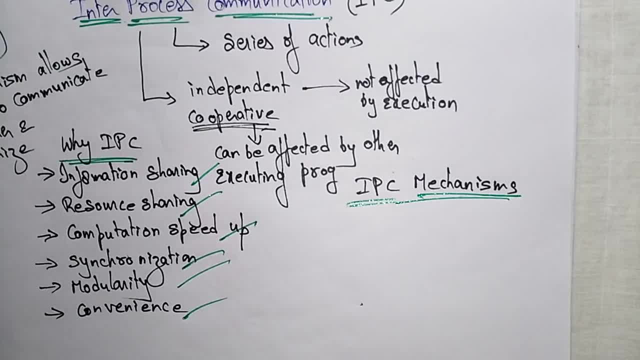 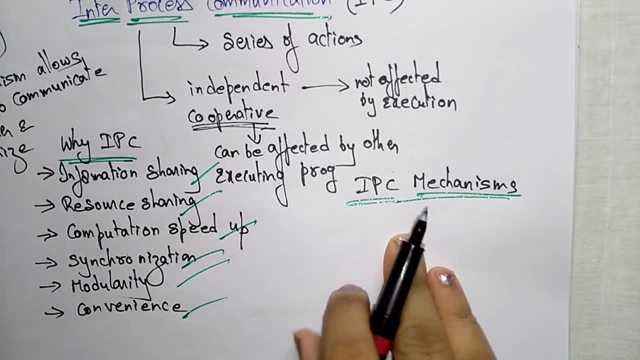 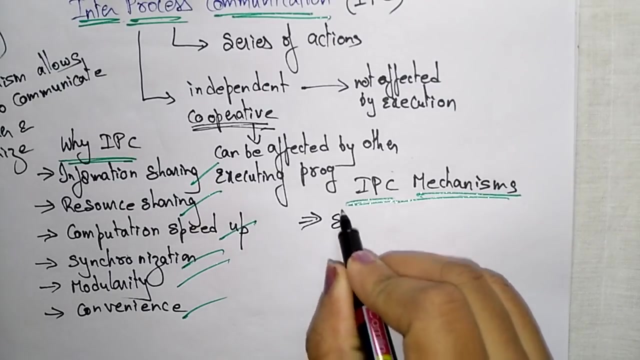 going for this mechanisms. so are Marty use seen that by via using inter process communication. so let us see the inter process communication mechanism. so here the process span each other by using two ways. in inter-process communication, the process can communicate with each other by using shared memory. shared memory and. 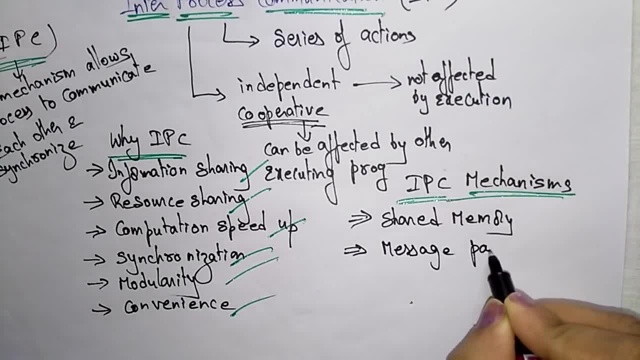 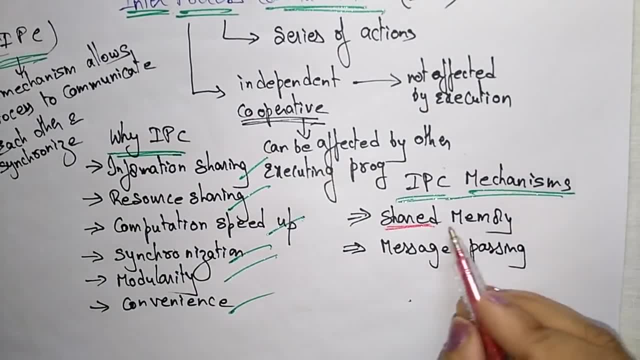 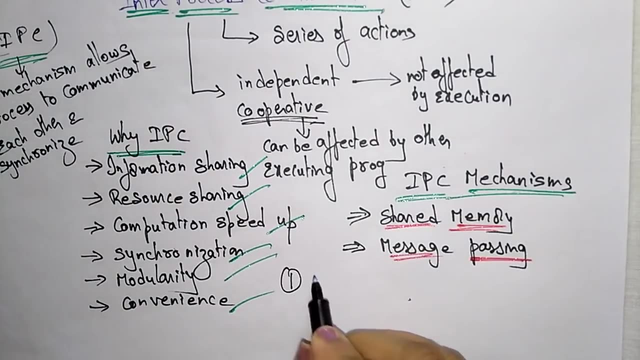 message passing. okay, so these are the two mechanisms that are used in the inter-process communication. so shared memory and message passing. so let us see one by one. so first will be the shared memory. okay, so shared memory here. let us take one diagram in the shared memory. 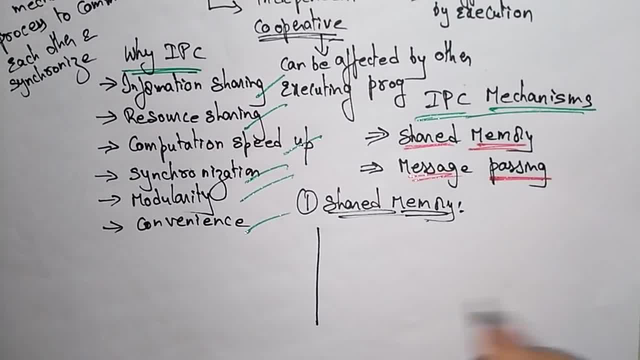 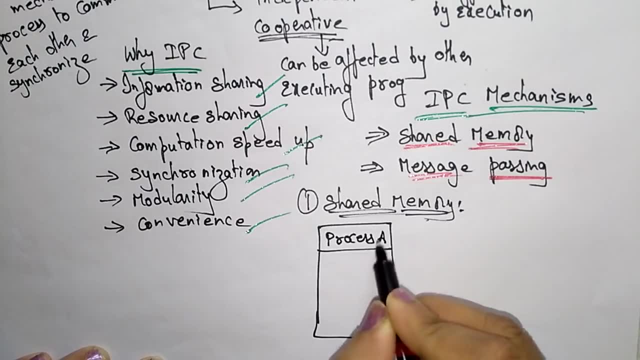 so this is here in one system. this is a process A, some shared memory is there. process B and some kernel. kernel is nothing but an operating system, whatever we using. so here the process where we'll share the data by using, with the help of shared memory and message passing. so let us see one by one. so let us see one by one, so let us. 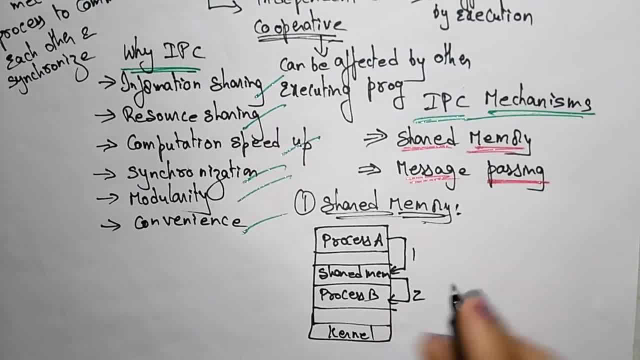 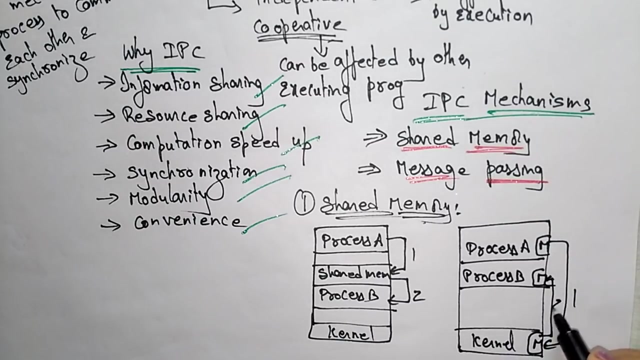 memory. that will content to so and this is another shared memory diagram. so here the process a, using a memory, and in the process B also you are having memory and this is the kernel. kernel is having the memory. so here this first communicate with the operating system. then it sends that message to the process B. okay, so 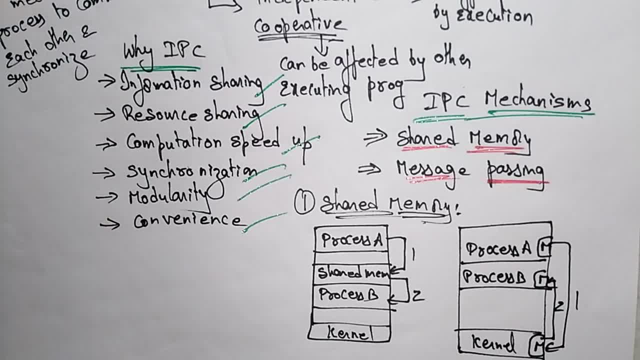 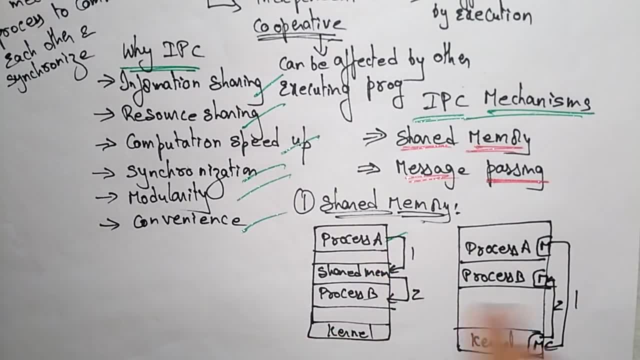 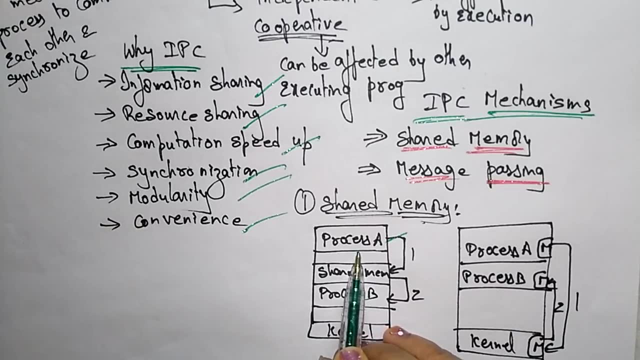 this is the shared memory here, process a. so this is the process a. so this process a generates information about certain resources. so, whatever the resources it wants to be used, it generate information about that resources and keeps it as a record in the shared memory. so it keeps it in. 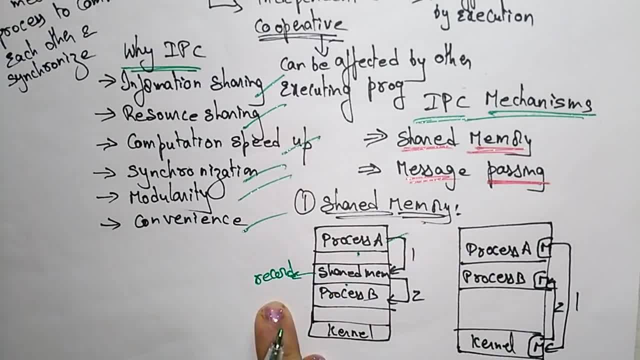 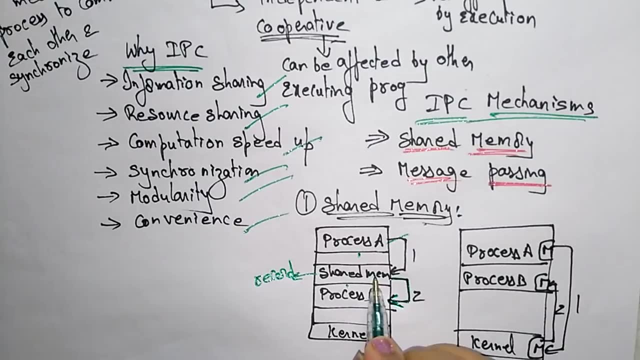 a record, a particular record, so in that record a resources that are used by the process a will be saved in the shared memory. okay, so when process B needs to use shared memory, suppose this process B wants to use the shared memory. so first what it does, it first check the record, whatever already present in the shared 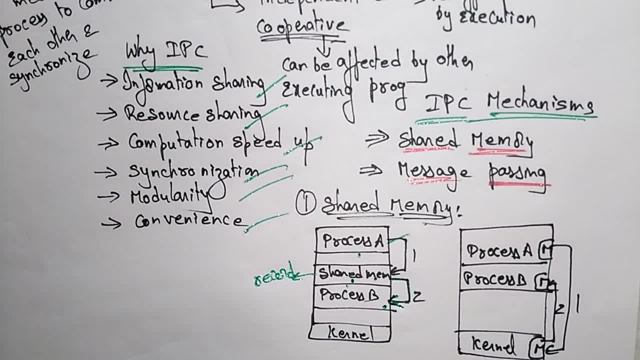 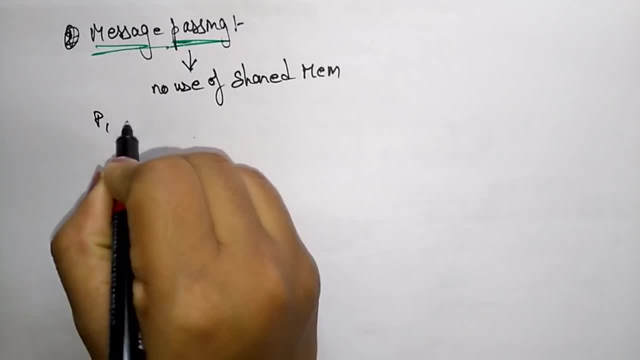 the shared memory will be saved in the shared memory. so, whatever the data that is used in the shared memory will be saved in the shared memory. so, whatever the data that is used in two process will be there, P1 and P2.. Suppose, if these two process wants to be communicate. 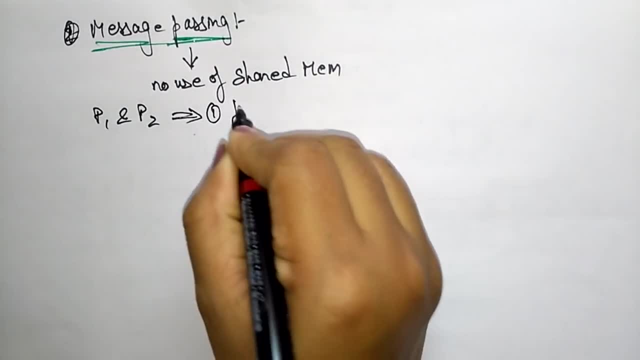 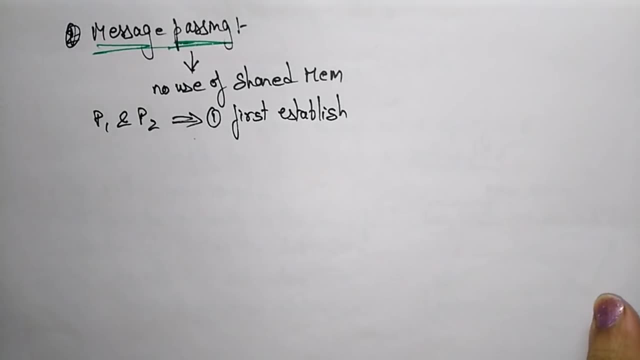 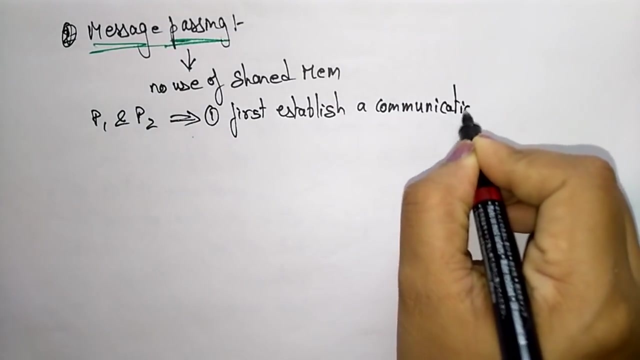 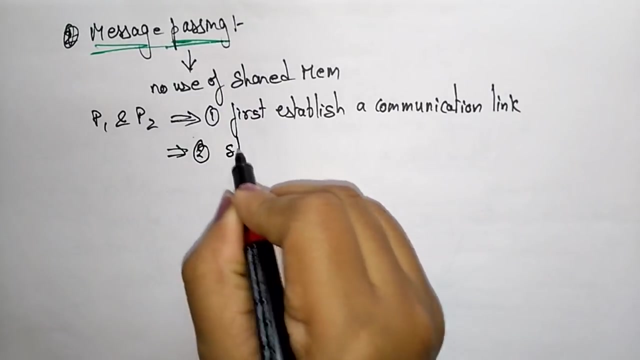 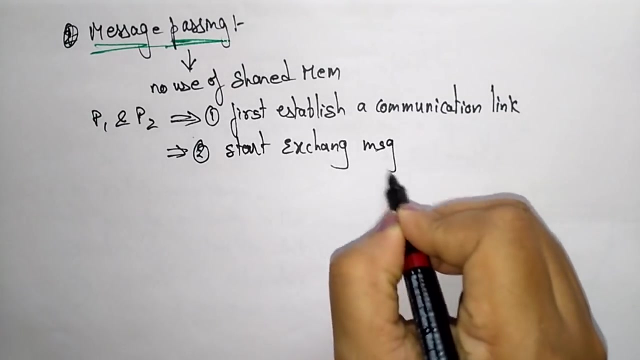 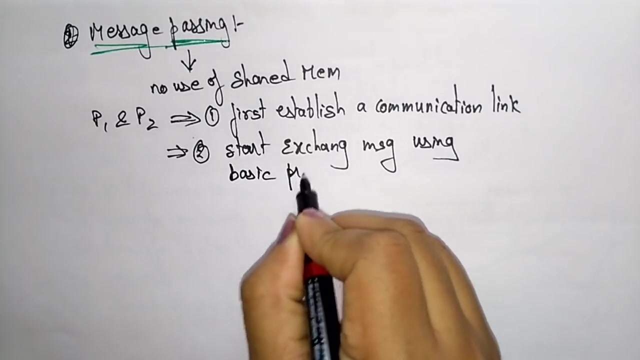 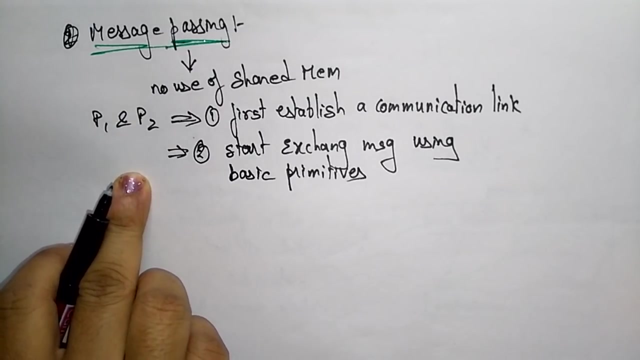 so what first they have to do? first, establish the first, establish a communication link. first, establish a communication link. second, what it has to do: it has start exchanging exchange message using basic primitives. okay, so if this two process, p1 and p2, wants to communicate to each other, first it has to establish a communication link. 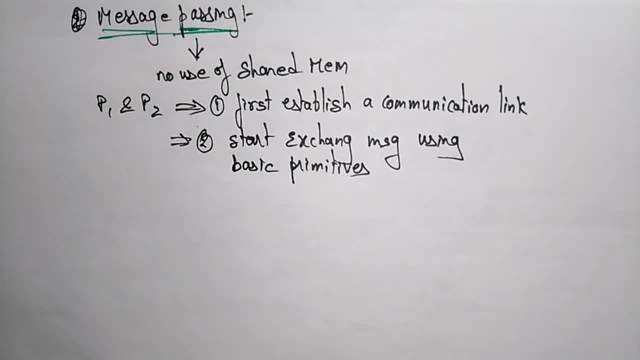 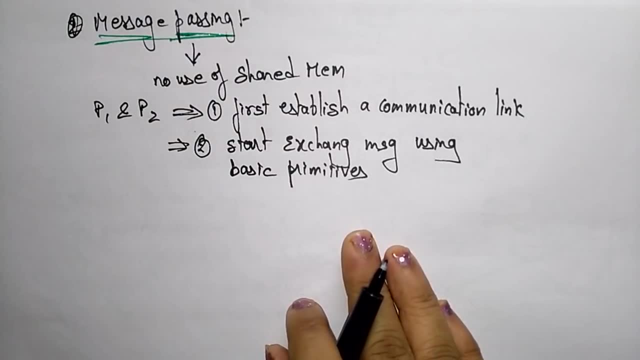 suppose if already the link is established, no need to again establish. once it is established it will be set. so second thing is it has to start exchange message using a basic primitive. so those primitives are the send and receive. so these are the two basic primitives that are used in the 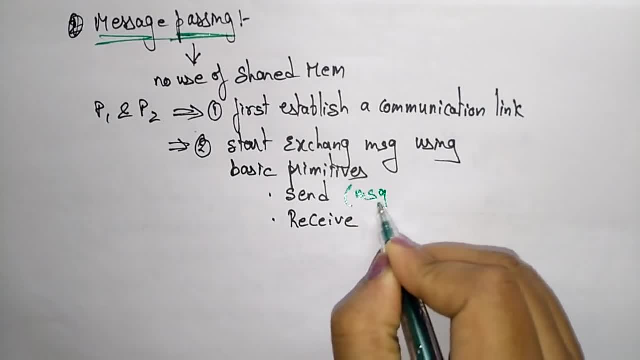 message passing send means while sending it has the send primitive is having message as well as destination to where it has to be sent. so whatever the message that it has to be sent, that message and the destination address has to be there in the receiving message will be there as well as. 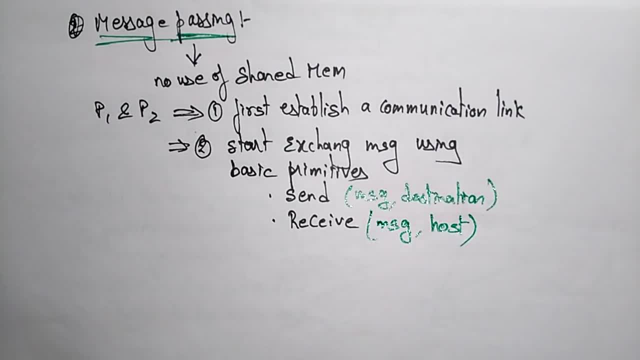 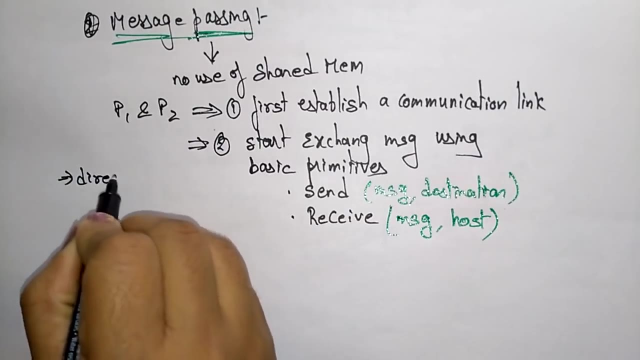 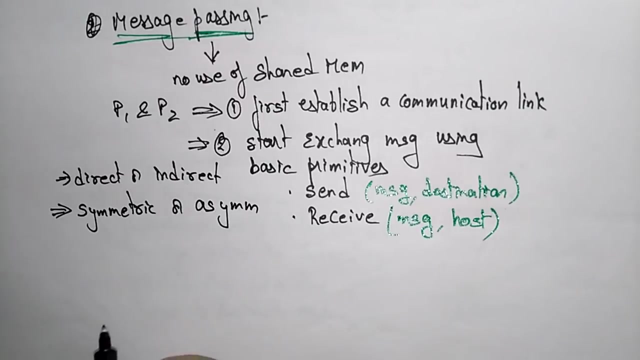 the host from where the message is coming. okay, so these are the two primitives that are used in message passing: sent and receive. so So this message passing may be a direct communication, it may be a direct or indirect communication. Okay, so next, it may be a symmetric or asymmetric communication, or it may be automatic or explicit. 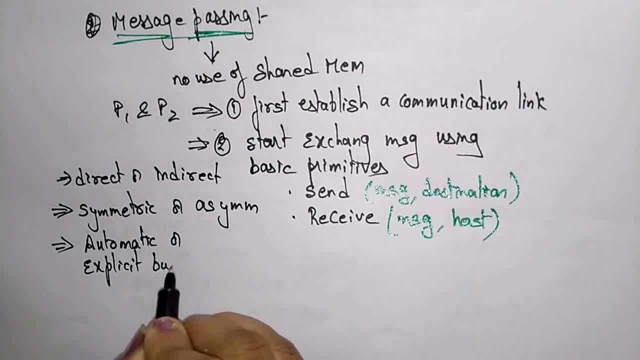 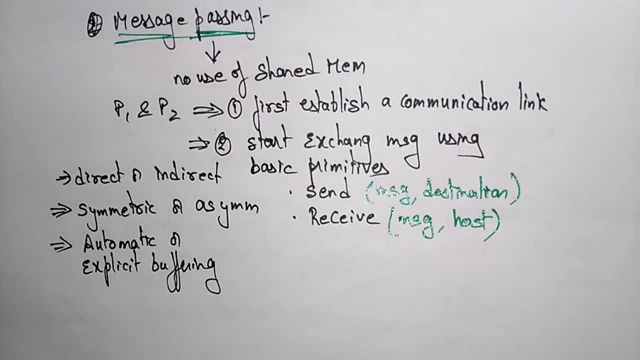 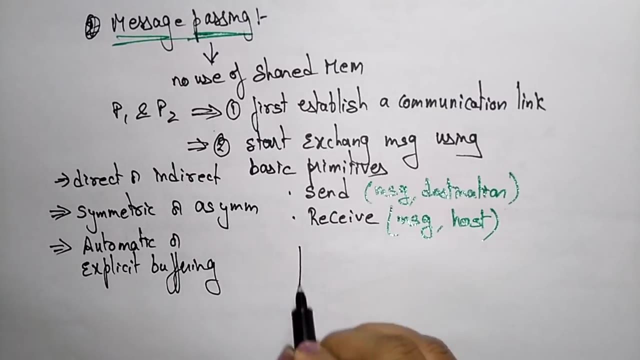 buffering. So this message passing may be, it is a direct or indirect, symmetric or asymmetric, or automatic or explicit buffering. So let us see: here This is sending process, So sending process required. So whatever it is sending, the message passing module And here what it is passing. 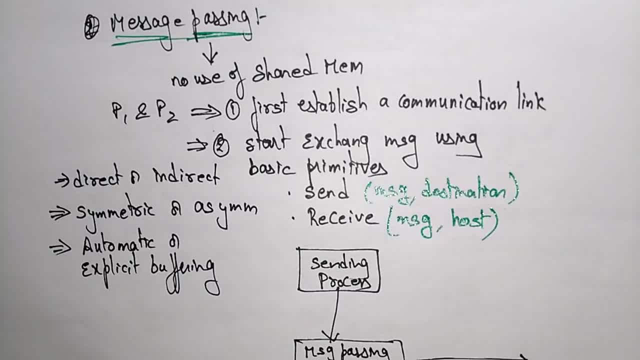 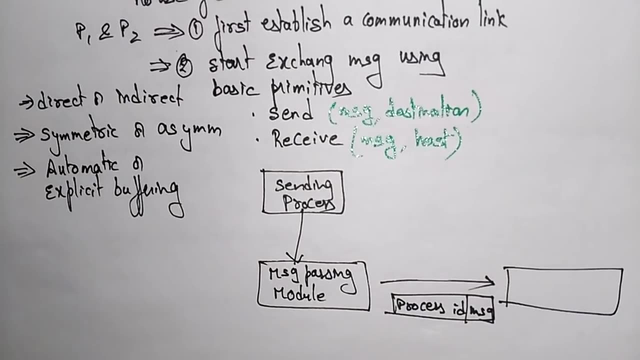 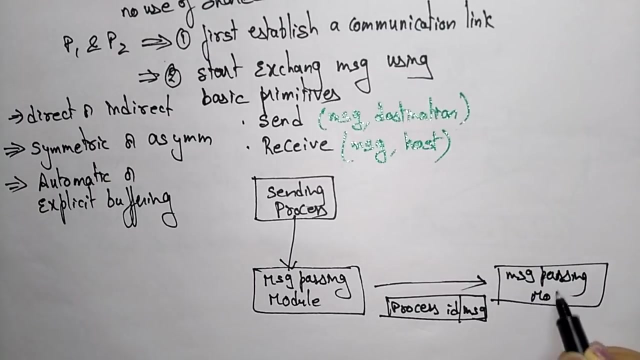 It is passing process ID and message. So, whatever the process ID means the ID and to where it has to be sent, that process ID and the message is passing From here it's having the message. Okay, So this is the way how the message is passing module.